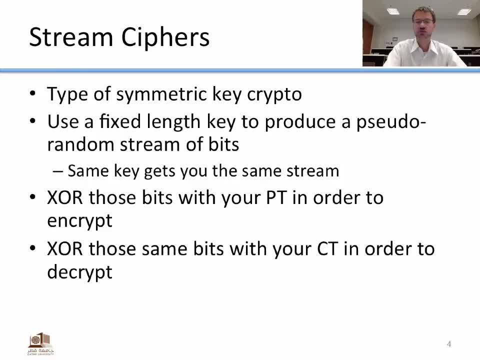 it works the same way. either way, whether you encrypting or decrypting, you're just exclusive or-ing your message with the bits from the bit stream. The goal of a stream cipher is to approximate a one-time pad. So when we discussed a one-time pad, I mentioned that it was the 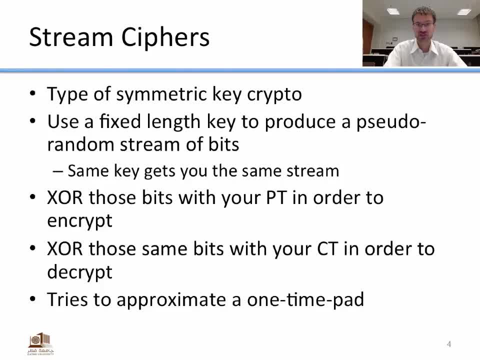 only provably secure form of cryptography, which is where your key is just as long as your message. Well, a stream cipher has the goal to approximate that, but instead of using a key that's as long as a message, you use a much smaller key, and then that key is used to generate a very, very, very long. 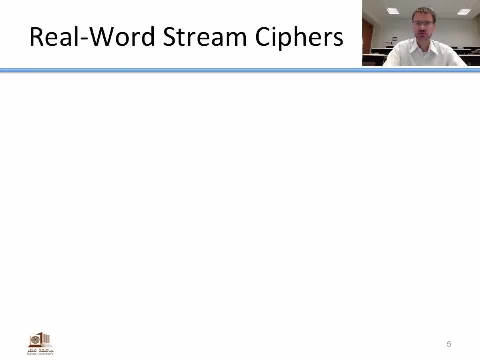 stream of bits. So let's look at some- two real world stream ciphers. The first is called RC4.. RC4 was a stream cipher that's most famously used in WEP- the wireless equivalent protocol-- wired equivalent protocol- for wireless. 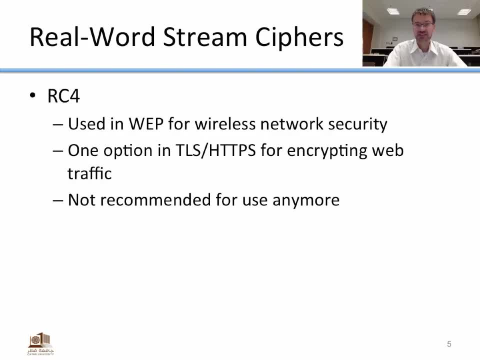 network security. It's also an option in TLS or HTTPS for encrypting web traffic, but it's not recommended for use anymore. It has some mathematical weaknesses that mean it's may- it's not suitable for quite a few applications. Another real-world. 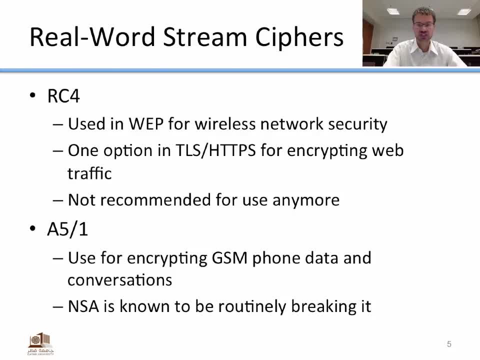 is A51. And this is used for encrypting GSM phone data and conversations, And so it's used to encrypt data before your phone sends it wirelessly to the operator. The NSA is known to routinely break A51. This was released as part of the Snowden leaks, So again it's another stream. 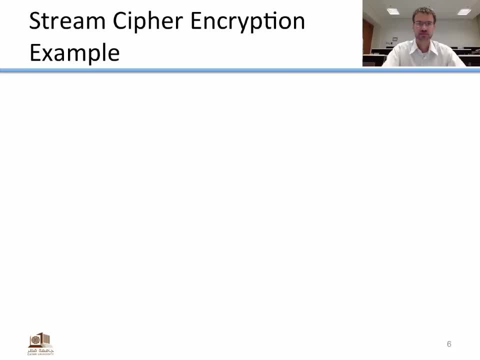 cipher. that's not really recommended for usage. So let's do a stream cipher encryption example. So let's say we have some plain text data that we want to encrypt And we have a key that we're going to use- In this case I'll just make it 128 bits- We take that key and we feed it into our 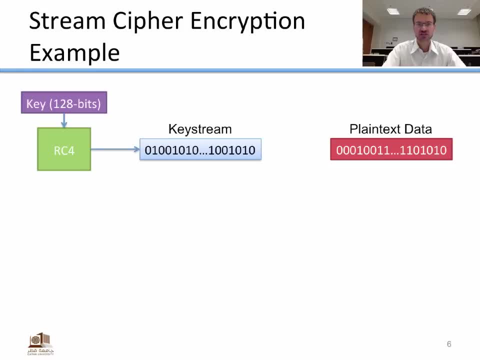 stream cipher, which in this case is RC4. And that causes RC4 to produce key stream, which is a potentially infinitely long string of ones and zeros. But we produce enough key streams so that we have the same length of key stream as we do plain text data. And then we exclusive or those. 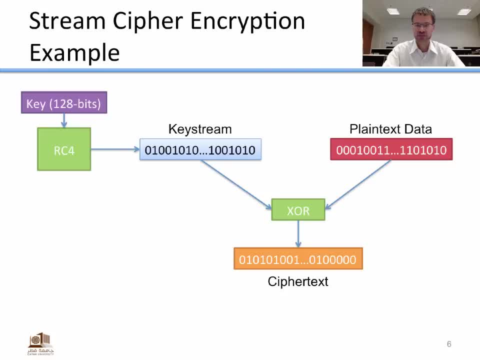 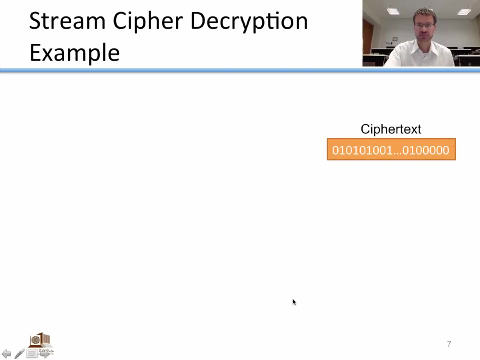 two things together in order to get our cipher text. So the key stream exclusive word with the plain text gets me the cipher text. So I could write that as cipher text equals the key stream exclusive word with the plain text. Well, how do I decrypt? Decryption is very similar, except in this case I have cipher text that I want to. 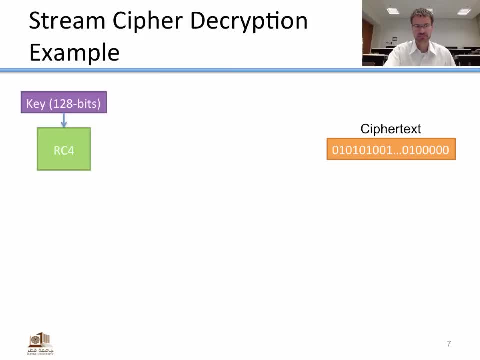 decrypt And I take that same key that was used to encrypt it. I put the key into RC4. I get out the same key stream that the person who encrypted got And when I exclusive or the key stream and the cipher text together, I get the plain text. Another way to write that would be to simply say that: 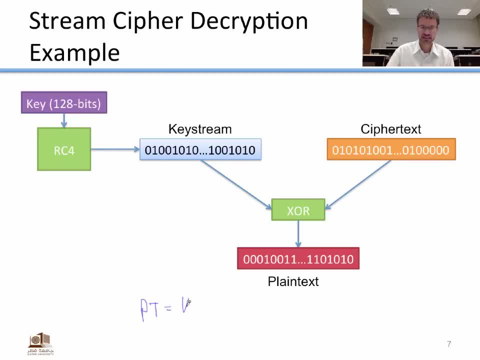 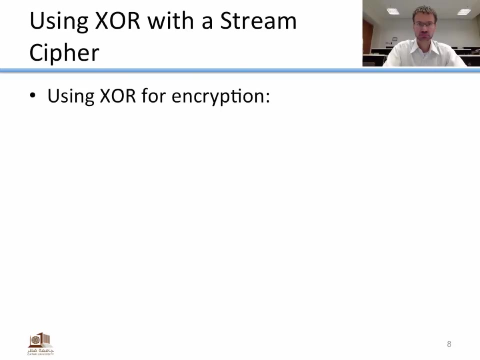 plain text equals key stream. exclusive word with cipher text. So let's look at that a little bit more about how we use exclusive or with a stream cipher. Now when we use exclusive or for encryption, we see that the cipher text equals the plain text. exclusive word with the key stream. 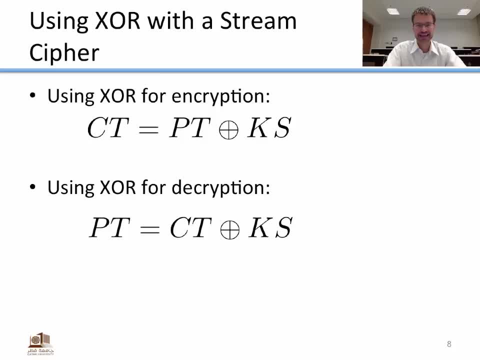 which is just what we went over. When we use it for decryption, the plain text equals the cipher text- exclusive word- with the key stream. So basically, whether you're encrypting or decrypting, you simply take the message you're working with and you exclusive, or it with the key stream, and that performs the 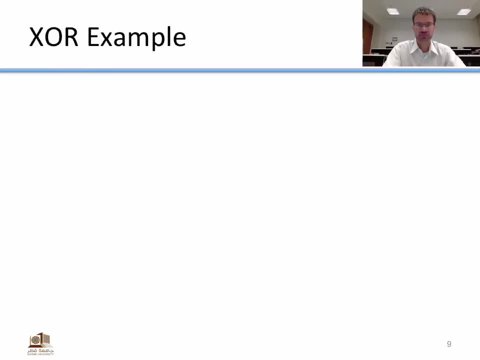 encryption or the decryption operation. Let's look at an example. So if I'm going to do an encryption and my plain text is here 0110. And my key stream is 1101. I'm going to exclusive or them together to get the cipher text. 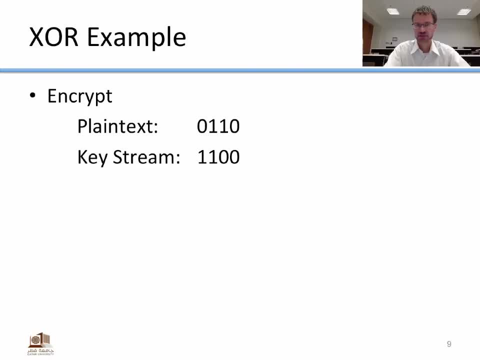 Now, in case you're not familiar with exclusive or or you've forgotten because it's been a long time since you've looked at it, here's the truth table for exclusive or, And what this shows is that if we exclusive or 1 together with 1, we get 0.. 1 exclusive or with 0 is 1., 0 exclusive or with 1 is 1.. And 0 exclusive or with 0 is 0.. 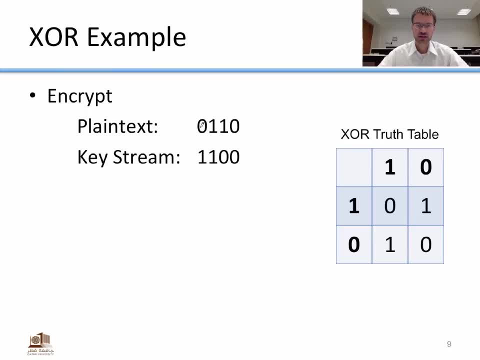 It's just the truth table for exclusive, or So if I look here and I see that the plain text is 0110, the key stream is 1101, when I do the exclusive or I'm just going to do it bitwise, 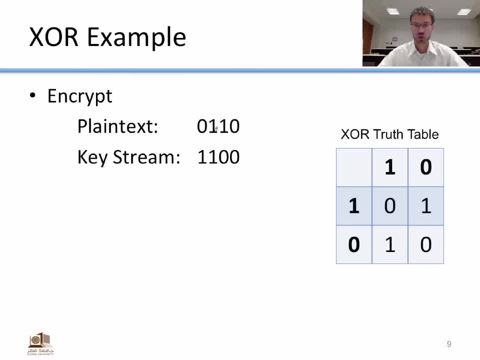 So 0 exclusive or with 1 is 1.. 1 exclusive or with 1 is 0.. So I have 1, 0.. 1 exclusive or with 0 is 1. And 0 exclusive or with 0 is 0.. 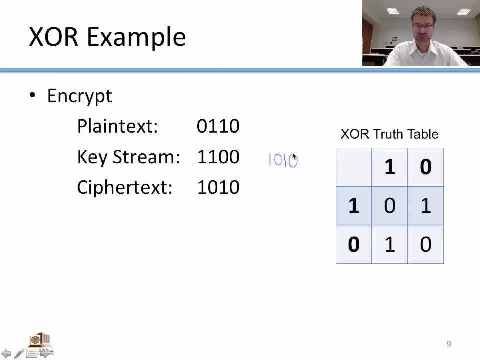 So my cipher text is 1010.. If I go to decrypt, then if I decrypt that cipher text using the exact same key stream, then I'm just going to exclusive or those together again. So 1 exclusive or with 1 is 0. 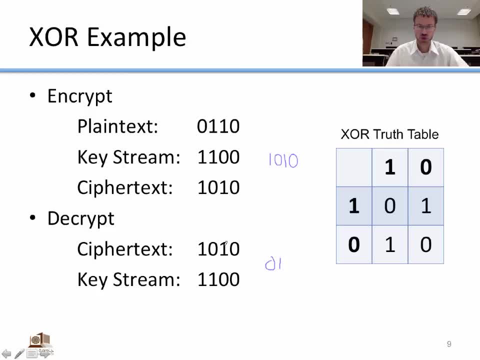 0 exclusive or with 1 is 1.. 1 exclusive or with 0 is 1., And 0 exclusive or with 0 is 0. So I get that result to be 0110.. And they match. So you can see up here that the original plain text I started with. 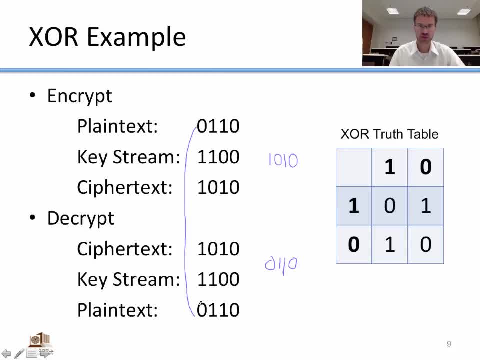 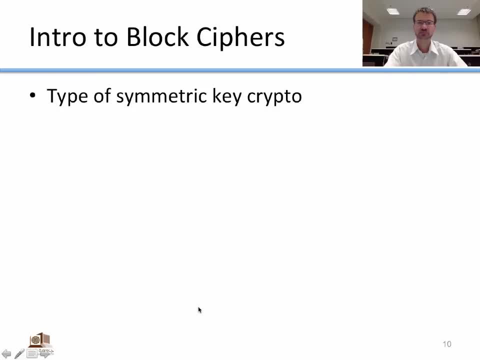 matches the plain text I get at the end when I decrypt. So I encrypt by exclusive or-ing with the key stream and I decrypt by exclusive or-ing with that same key stream. So that was stream ciphers. Now we also want to look at something called block ciphers. 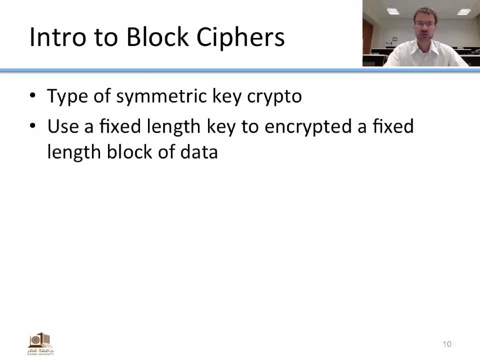 Now, block ciphers are another type of symmetric key crypto And what they do is they use a fixed length key to encrypt a fixed length block of data. So a stream cipher generated key stream and you exclusive or-ed that together. a block cipher encrypts specific blocks, fixed length chunks of data. 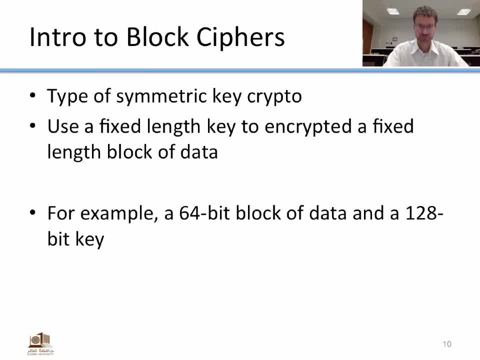 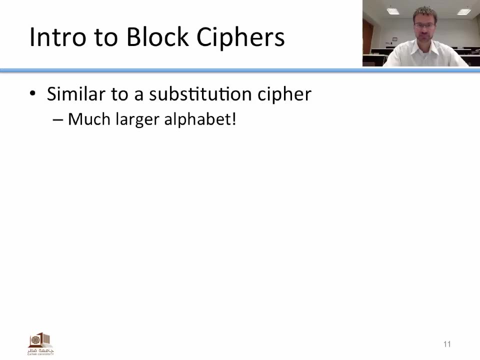 into a ciphertext of the exact same length. So, for example, a 64-bit block of data and a 128-bit key could be the parameters for a block cipher. So I could have a block cipher where my key is 128 bits and I encrypt 64 bits of data at a time. 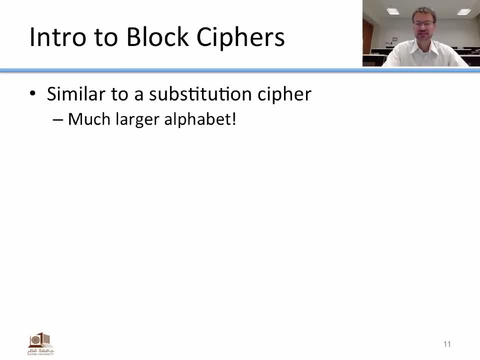 Now at its core. a block cipher is in some ways very similar to a substitution, But with a much larger alphabet. So remember, in a substitution cipher we simply had every letter written out as one entry in a table and then we randomly permuted the entries. 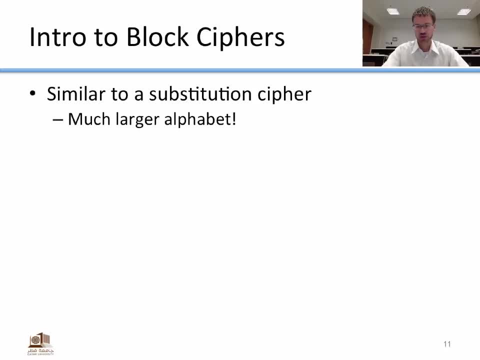 so that the encrypted version was just a randomized list of the alphabet. So that meant that every letter in the plaintext had a one-to-one correspondence with a letter in the ciphertext. A block cipher is basically the same thing, except our alphabet size is a lot bigger. 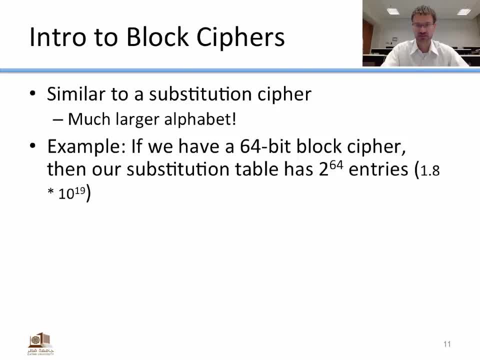 instead of it just being 26 bits. It's every possible, say, 64-bit value. So if we were to do a 64-bit block cipher, that would mean that our substitution table would have 2 to the 64 entries. 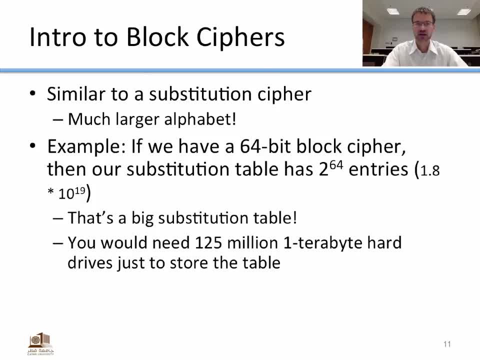 which is 1.8 times 10 to the 19. That's a huge number. That would be a really big substitution table. In fact it would be 125 million terabytes, So it's huge. So I don't give this example to say that this is how a block cipher works. 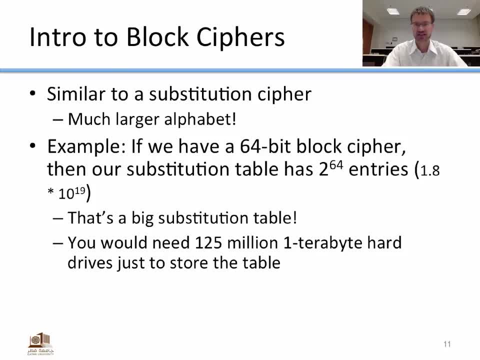 It doesn't build an actual table, But the idea is the same. in concept, Every 64 bits of plaintext would have a corresponding ciphertext for a given key. So my goal of a block cipher is to do this same thing, but do it with an algorithm and a small key. 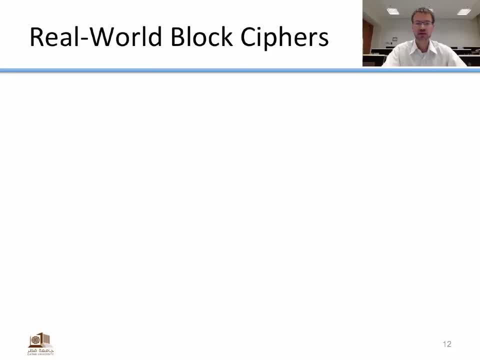 instead of building up an enormous table. So some real-world block ciphers. We'll go over two of them. The first is the Data Encryption Standard DES. DES was a US government standard until 2001.. It was released in 1976.. 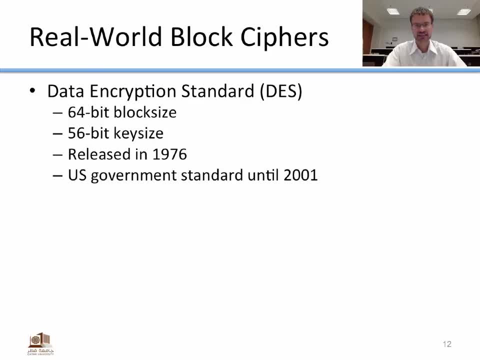 And it uses a 64-bit block size and a 56-bit key size, So the key was 56 bits, but the blocks of data that you encrypt are 64 bits. Now, DES was replaced by AES, the Advanced Encryption Standard. 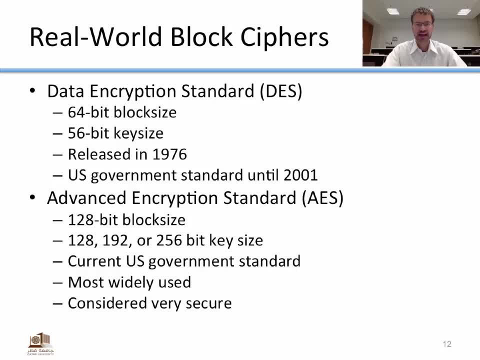 And AES uses a 128-bit block size And it can take a variety of key sizes, either 128,, 192, or 256 bits for the key size. AES is the current US government standard And it's probably the most widely used symmetric key algorithm in most applications today. 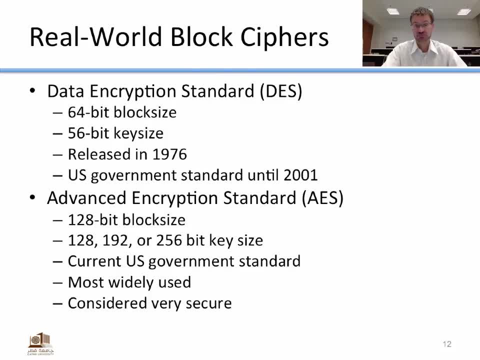 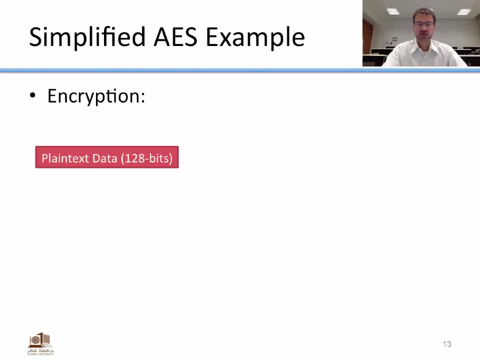 And it's considered very secure. Lots of smart people have looked at it and they haven't found any significant weaknesses. Let's do a simplified AES example, So in this case, my encryption. I take some plain text data of one block size. 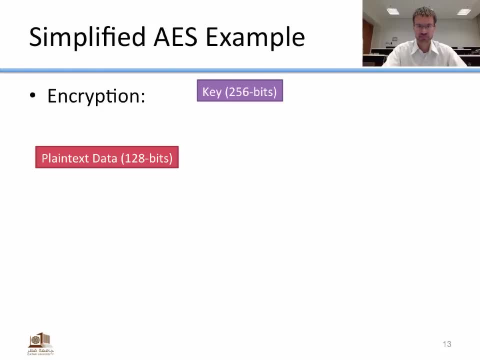 So if we're doing AES, that block size is 128 bits. I take a key which is 256 bits for AES here And I run it through the AES encryption algorithm So the key and the data go in together And that produces ciphertext data of 128 bits. 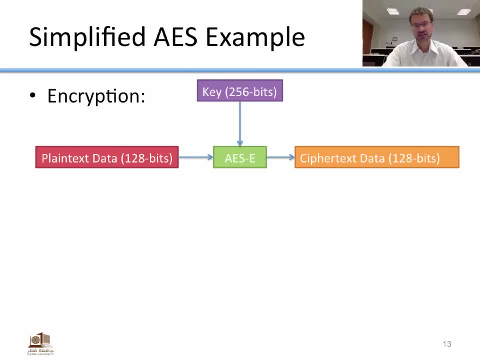 So my plain text block is converted to a ciphertext block of the same size And when I decrypt I do the same thing in reverse: I put my ciphertext and the key into the AES decryption algorithm And I get out the plain text data. 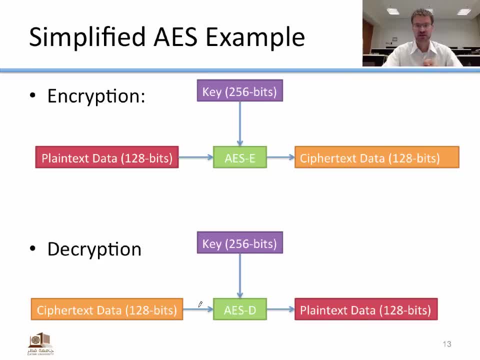 Now it's really interesting. It's really important to note a couple of things here. First is that the block size is really important. You can't use a block cipher to encrypt something that's smaller or larger than the block size. You can only encrypt an item that is exactly that size. 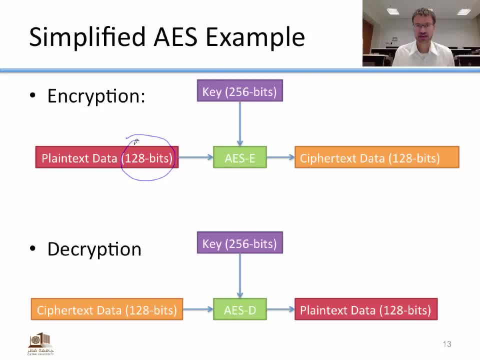 So if your item is smaller than, in this case, 128 bits, you would need to break it up into pieces and encrypt each piece separately. If your item is bigger than the block size- in this case, 128 bits- then you would need to break it up into smaller pieces. 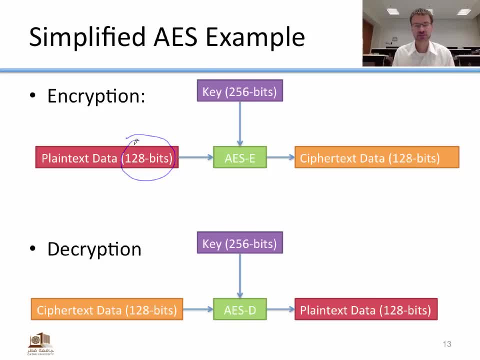 and encrypt each 128-bit piece separately. If your item is smaller than 128 bits, then you would need to add some junk. We call it padding. Just add some extra bits to get it up to the right size, Because a block cipher only encrypts chunks of data that are the right size blocks. 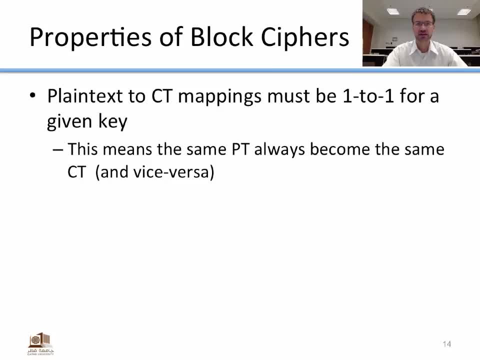 So let's look at some properties of block ciphers Now. one important property is that the plain text to ciphertext mappings must be one-to-one for a given key. So that means that for a given key the same plain text block always becomes the same ciphertext block. 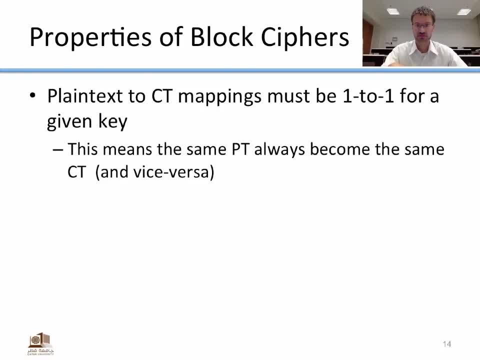 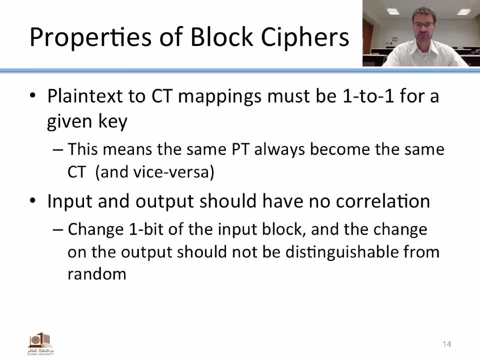 and the same ciphertext block always becomes the same plain text block, So vice versa. It's also really important that the input and output have no correlation. So what this means is, if I have a 128-bit input block, that will produce an output block. 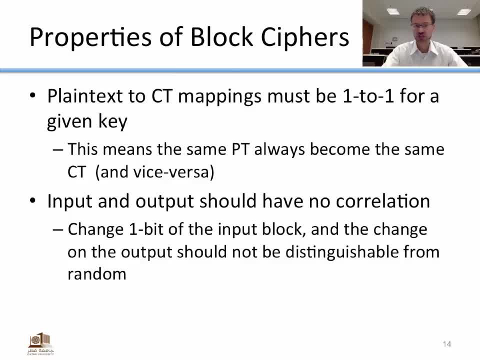 If I change one bit of that input block, then the output block should change significantly In a way that's not distinguishable from random- And not distinguishable from random is just a big fancy way to say that about 50% of the bits should change. 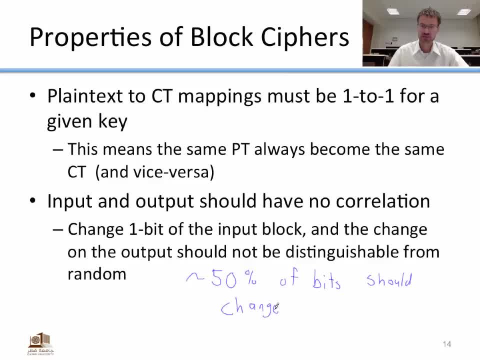 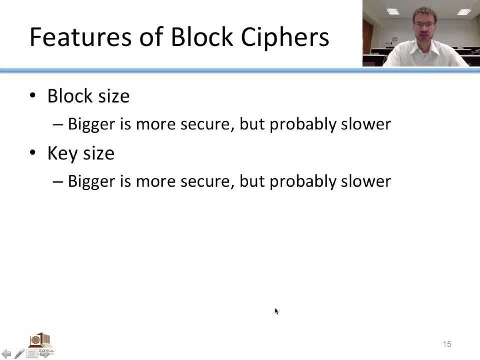 So if I change one bit on the input then about 50% of the output bits should change. Let's look at some features of block ciphers. The first is the block size In general. the bigger the block size, the more secure it is to an extent.